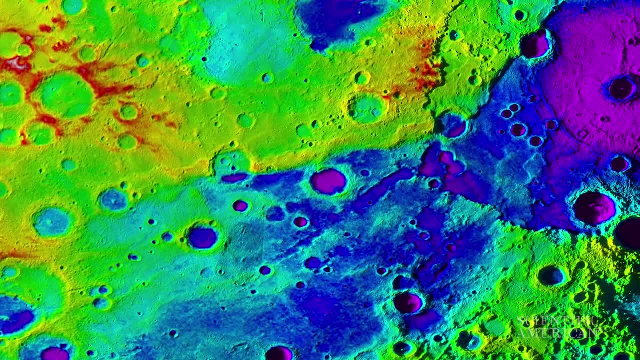 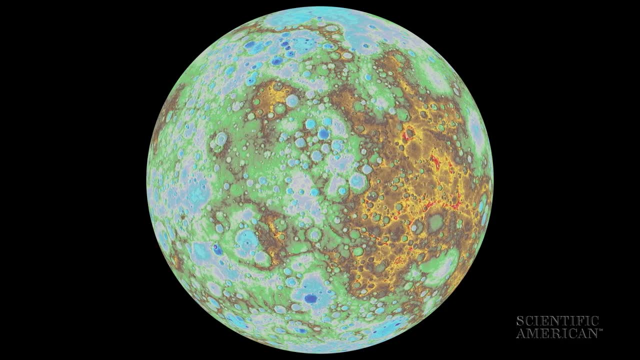 discovered a colossal canyon twice as deep as the Grand Canyon. Mercury is gradually shrinking, as it cools and as it shrinks. it crumples up like a grape, shrinks into a raisin and making those little crevices- except this is a really big crevice, Wild. Now Venus isn't shrinking, is it? 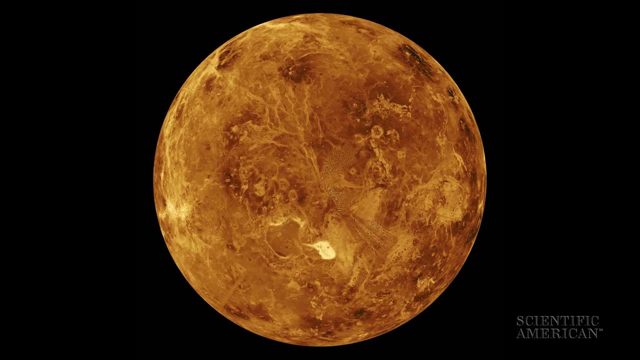 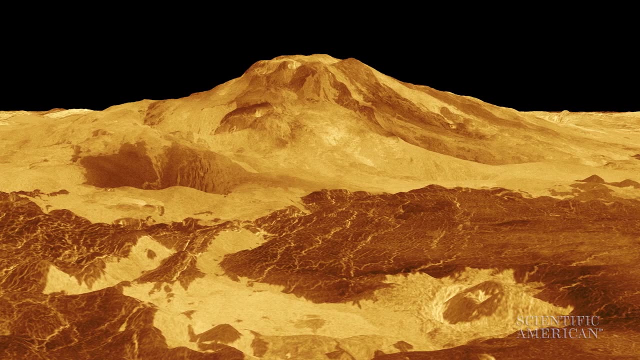 Venus is not shrinking, but it is showing evidence that it once might have had oceans where life could have existed before the temperature went up to 900 degrees, and life could still be persisting in the clouds and we could actually go look for it. 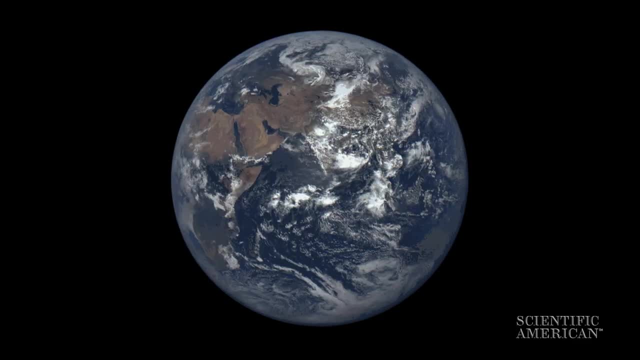 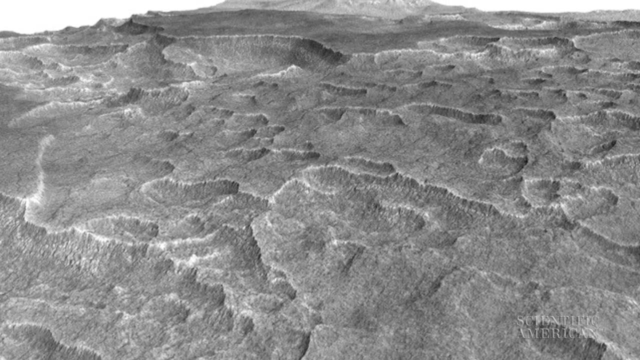 Okay, we're going to skip over Earth. I guess No one cares about Earth in the context of space, but leave it to Mars. Mars Reconnaissance Observer has discovered an ice sheet 560 feet thick and has as much water as Lake Superior. so if you ever get to Mars to live, you'll have a place to. 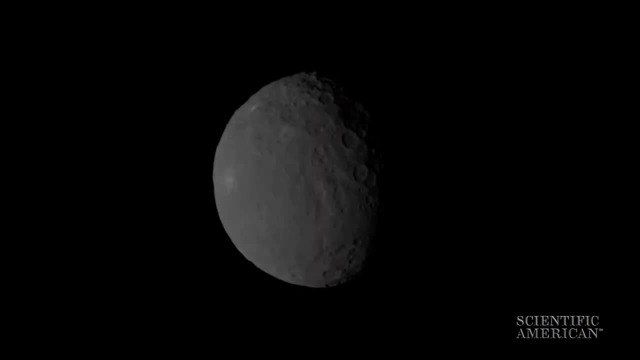 drink Man. that's kind of scary. It's seeming like a theme here, with water Moving on to the outer solar system. there's a place- the dwarf planet- called Ceres. There's water there too, it seems. We found actually what. 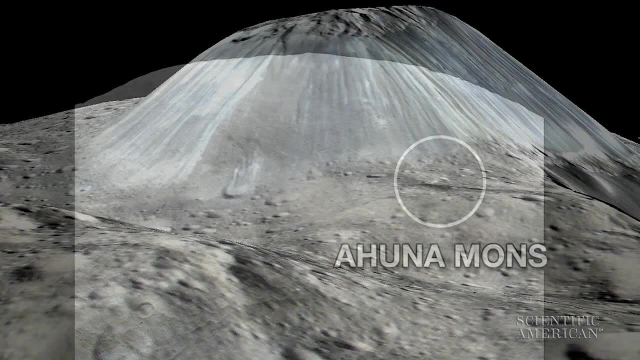 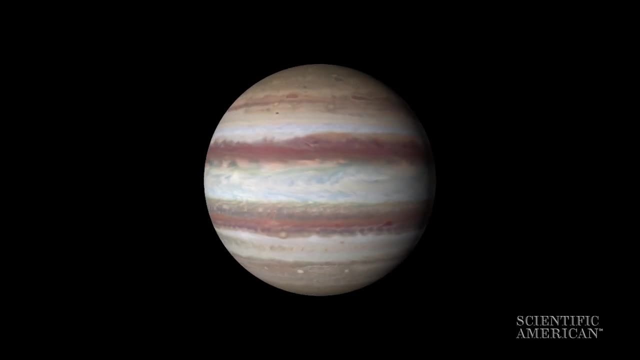 looks to be a cryovolcano, a volcano built from flowing liquid water rather than from flowing liquid rock. Pretty crazy, even though there's probably not an ocean there, But if we move to Jupiter, one of its moons called Europa, there does seem to be a subsurface ocean there. We've 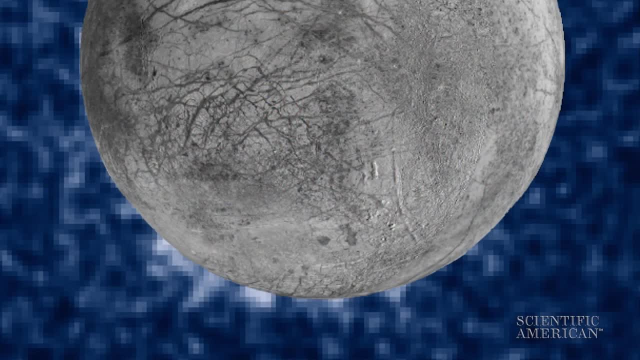 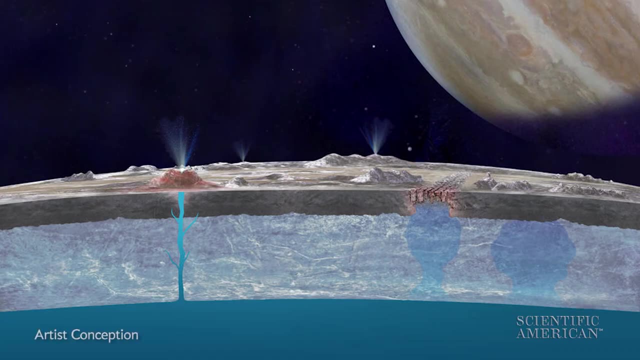 known that for a long time, but now it seems, based on new observations with Hubble, that there are plumes of water vapor emerging from this subsurface ocean, which is a good, good prospect for life and for us studying it. So the real news from Saturn is the end of news. 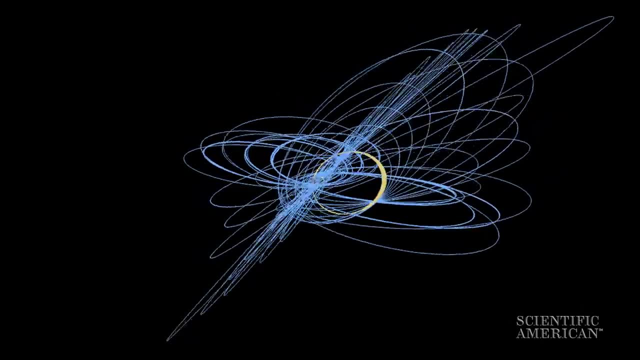 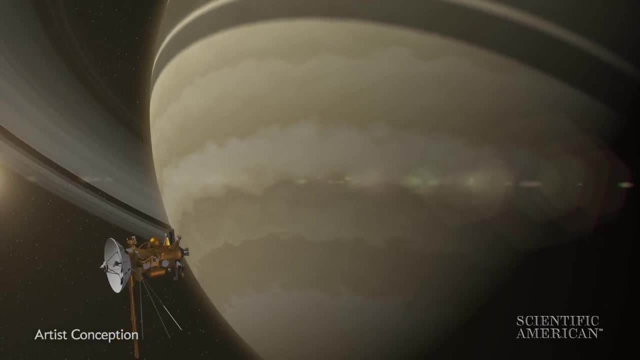 because the Cassini mission that's been there more than a decade is prepping for the end, changing its orbit, starting to dive through Saturn's rings, lining up for what's going to be a spectacular plunge into the atmosphere, September 15th of next year, when it will burn up. 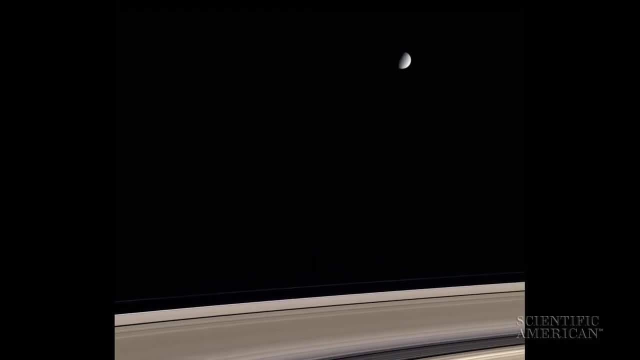 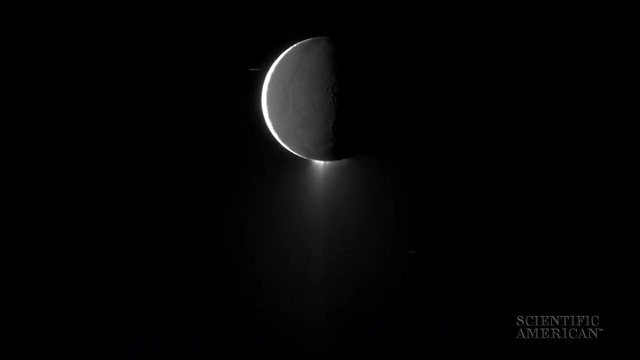 Yeah, they want it to burn up so it won't inadvertently crash into one of the moons and contaminate it. because there are a couple of moons, Titan and Enceladus in particular, where there's also evidence of underground oceans where there could be life, and we don't want to. 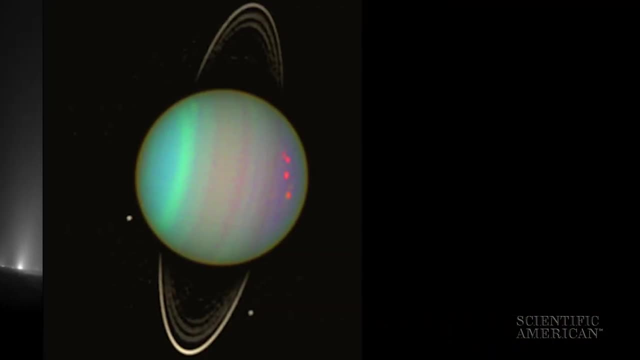 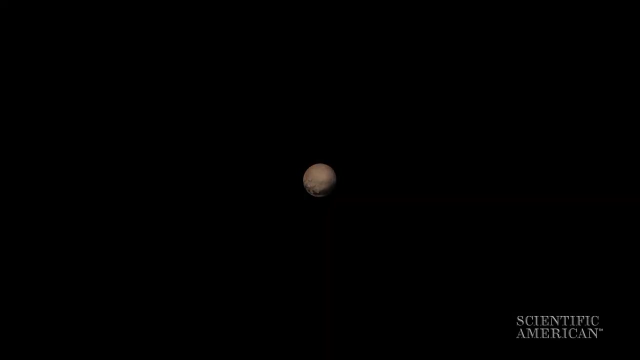 mess that up Yet more oceans in the outer solar system, which leads us to Uranus and Neptune. We don't really know much about them and we won't for some time, because there's no spacecraft there. Right On to Pluto. On to Pluto: We visited it last year with New Horizons and we've been.